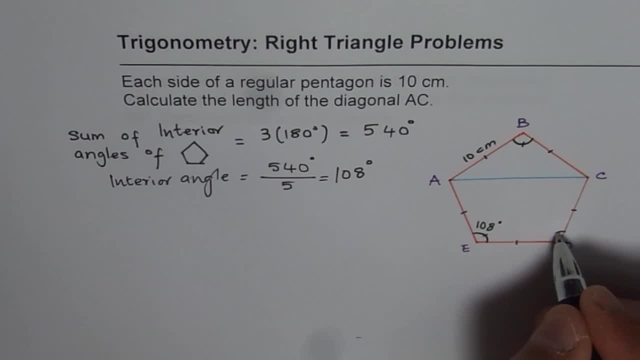 Correct. All these interior angles are 108 degrees each for a pentagon. Now to find the length of AC, what we can do is we can drop a perpendicular from B to the diagonal AC. So if I drop a perpendicular from B it is going to bisect AC, since both these sides are of equal length, right? 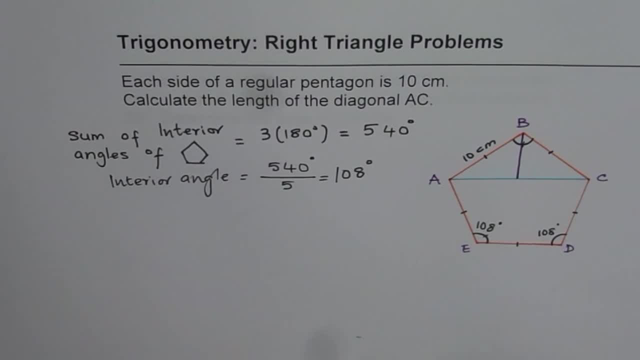 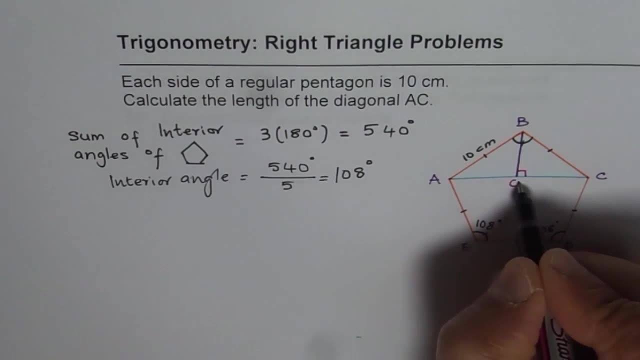 So if I have a perpendicular, perpendicular here from B, then this is a perpendicular. Let us say it is at point O, Then it is going to bisect AC. You can prove it, since this side is common. We have 90 degrees. 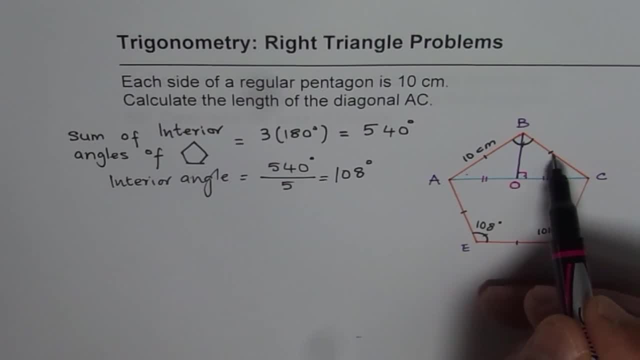 here, right? These two angles and the opposite sides are equal, right? So it is going to. so these two triangles are congruent. Since these two triangles are congruent, all their angles will be equal. Or in an isosceles triangle, whenever you draw a perpendicular: 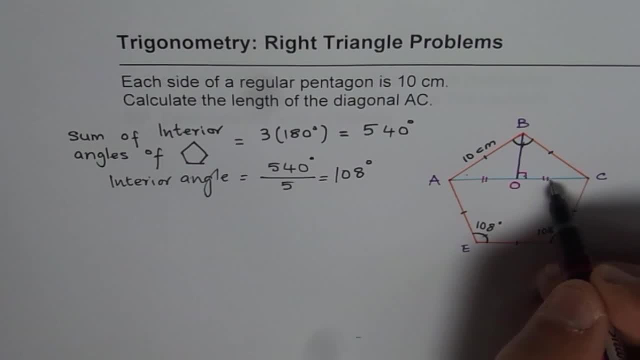 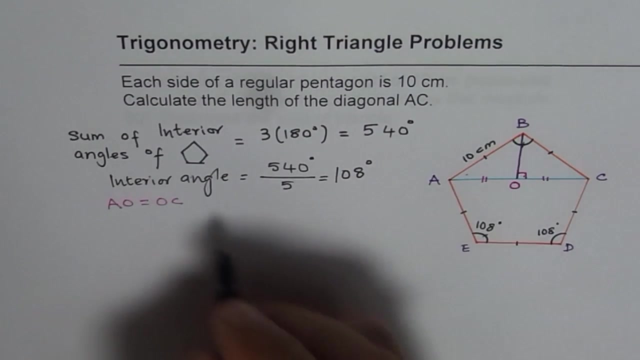 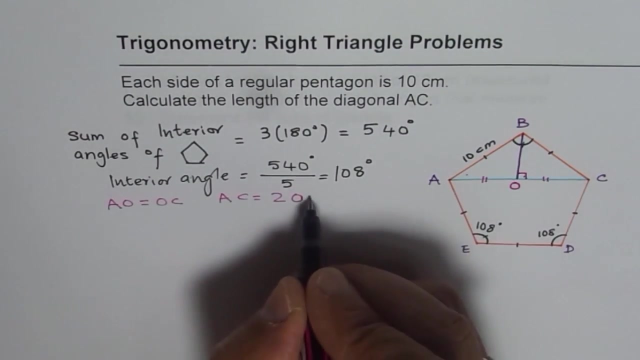 it will divide it into two congruent triangles. Their base will be same, So AO is equals to OC. Now we know AO equals to OC And AO equals to OC. AC is two times AO, correct? I can write OA now, So AC is twice AO. Now, if I can find, 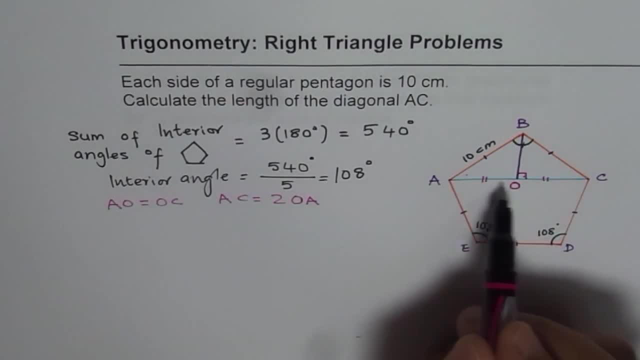 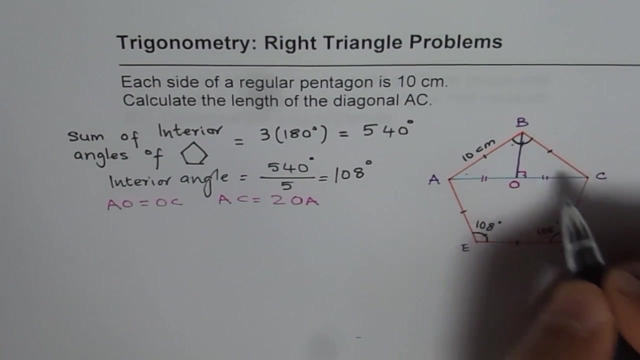 AO, I will find AC, since AO is half of the diagonal length AC. Now, how can you use your trigonometric? Now, how can you use the primary trigonometric ratios to find AO? We know this is hypotenuse, which is 10 centimeters for a right triangle. Now, this angle is half. 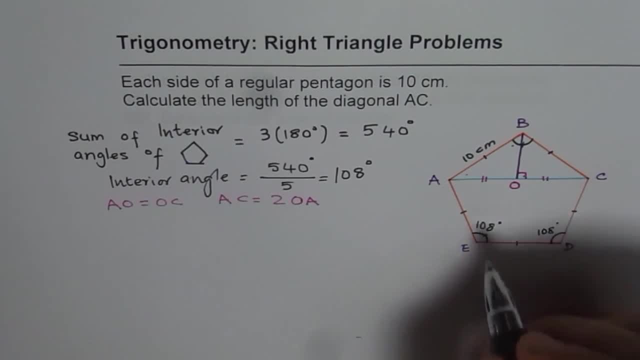 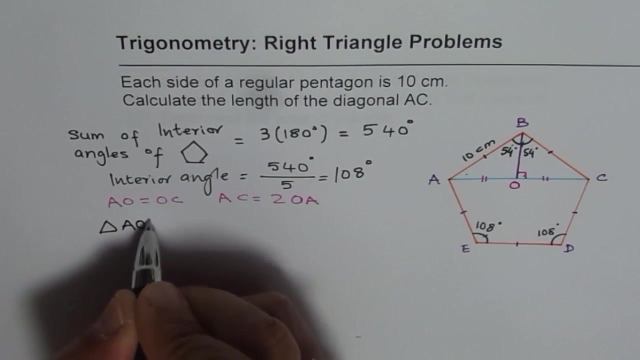 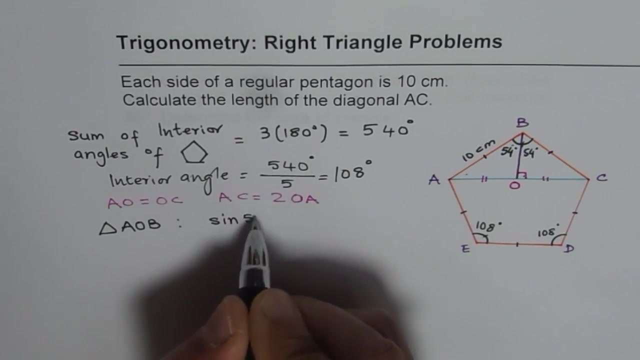 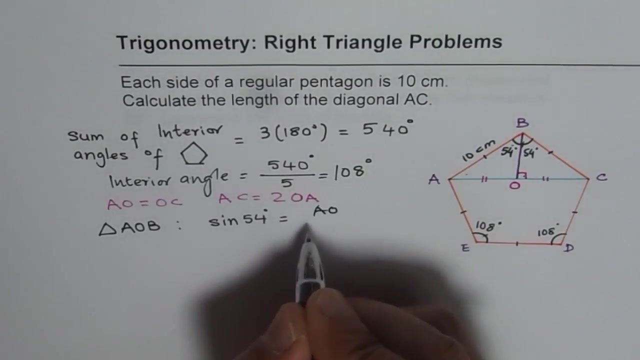 of 108 degrees. Half of 108 will be 54. So it divides into 54 degrees each. Now, if you look at the triangle AOB, let's consider triangle AOB, which is a right triangle. What is sine of 54 degrees? Sine of 54 degrees will be opposite side AO divided by hypotenuse. 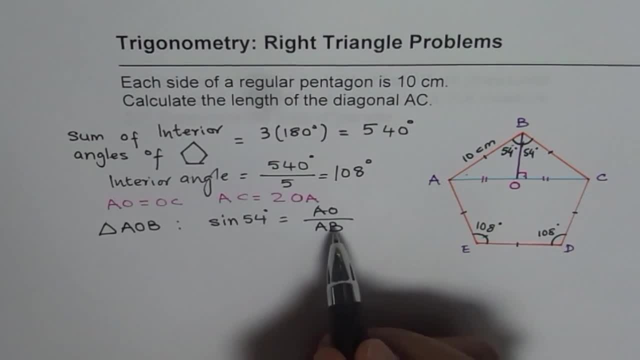 AB. Now from here we can find AO, right. So AO equals to length, AB times sine of 54 degrees. AB is 10, right. So we can write 10 times sine of 54 degrees. So we can calculate this using the calculator. So we have 54. 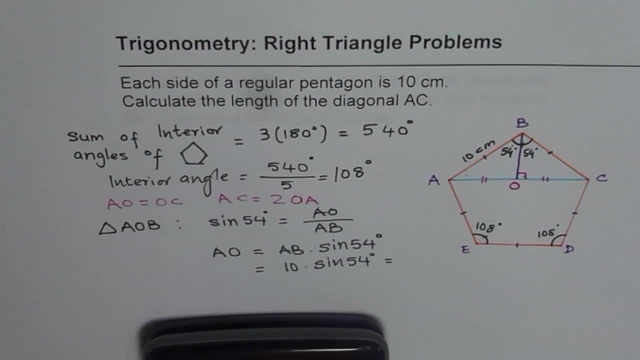 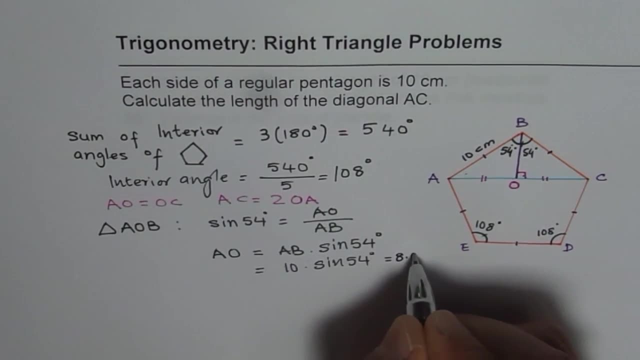 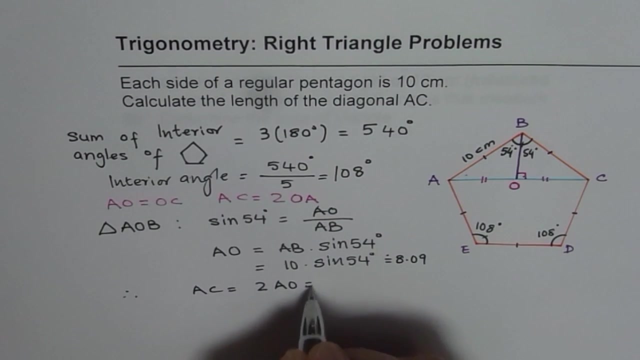 times, 10 times sine of 54, which is 8.0902.. Let me write this as 8.09 approximately, So we know AO is 8.09 centimeters And therefore AC should be equal to 2 times AO, which is: 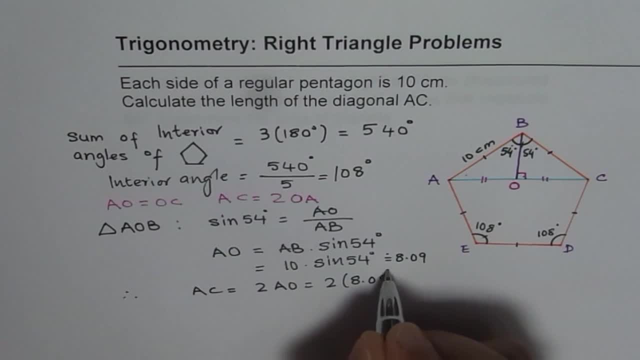 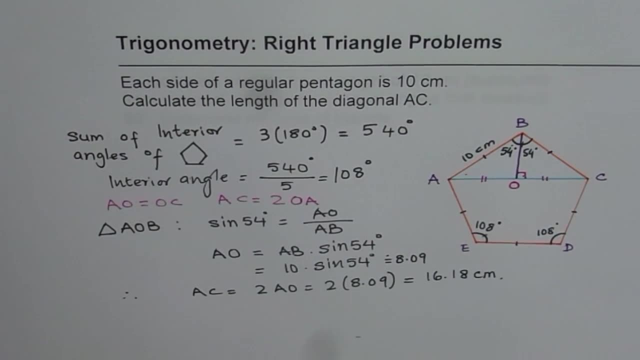 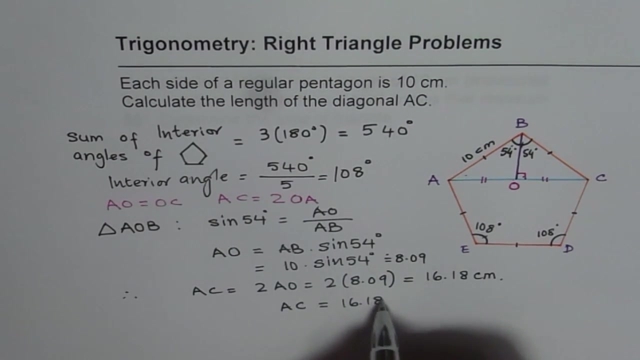 2 times 8.09.. gives us 16.18 cm. So our answer is that the diagonal AC is equal to 16.18 cm. So let's look back how we solved it. Since it's a regular pentagon means all sides are. 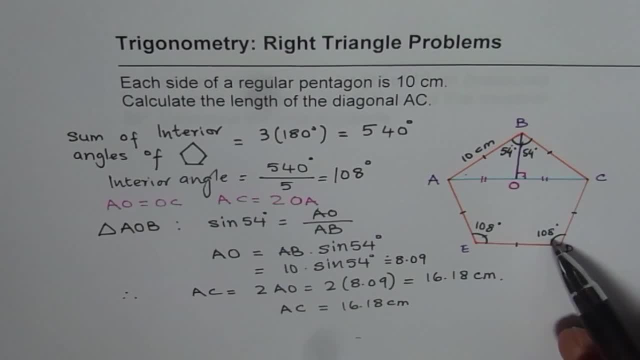 of equal length. all interior angles are of equal dimension. we can find interior angles by knowing that sum of interior angles for a pentagon is 3 times 180, which is 540.. Each angle should therefore be 540 divided by 5, which is 108 degrees. If I bisect the angle. 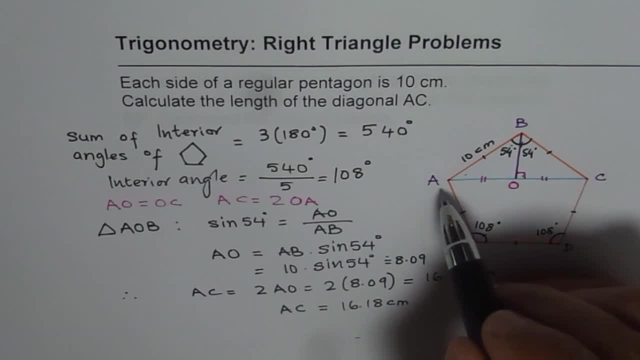 or if I drop a perpendicular from B to AC, it is going to bisect the angle at B. If I into 54 and 54, since these two triangles are concurrent. Knowing the angle and the hypotenuse, we can find the opposite side using sign ratio, the trigonometric ratio. sign of 54. 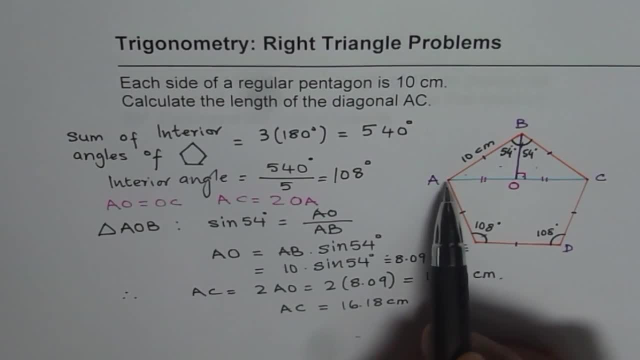 So we can use sign of 54 and find half the diagonal length, and twice that length will give us the required length of the diagonal AC. So that is how we can solve this question. I hope you understand and appreciate it. Thank you and all the best.